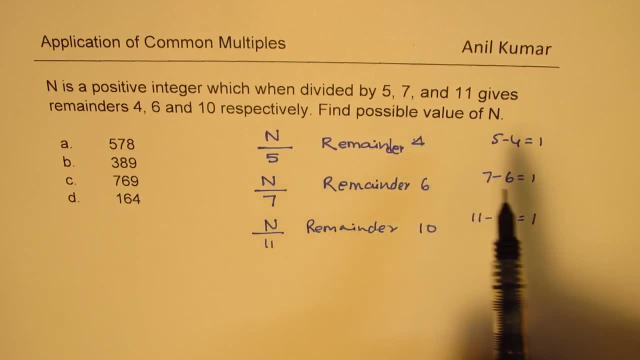 That shows you what It really means that we are looking for a number which is 1, because, see, when you divide N by 5, then what remains is 7, and 11 is also 1.. We are going to see a higher number, and if you divide N by 4,, then what remains is 7 and 11, and 11 is also 1.. 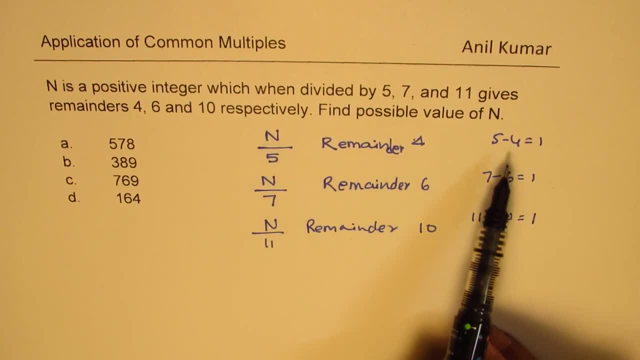 So N is a positive integer. When we divide N by 5, then what remains is 7 and 11, and 11 is also 1.. see, when you divide by 5 and get a remainder of 4, that really means that the number is 1 less than 5 right, 5 multiple right. so that means the number. 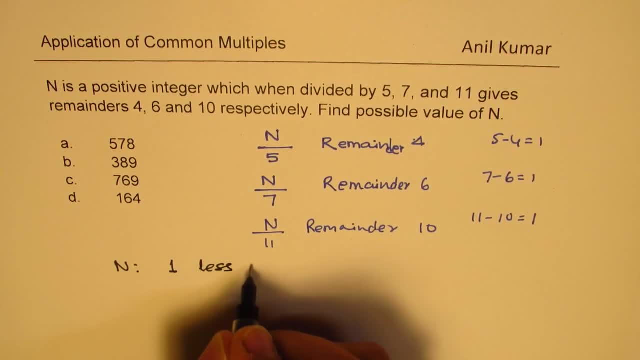 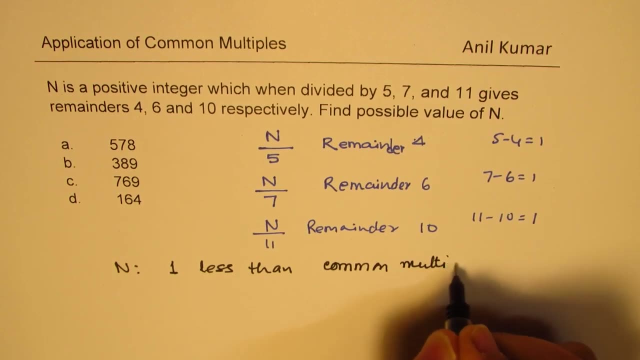 n is 1 less than common multiple, or these divisors which are 5, 7 and 11. you get the idea. so if I have a number which is a multiple of these numbers, then that will give you no remainder. however, the remainder is going to be less than 1. 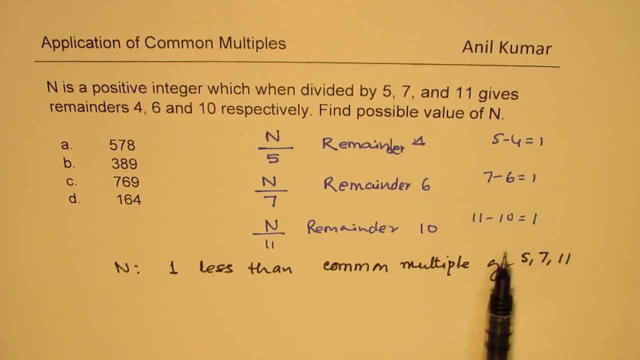 less than the divisor only when this common multiple minus 1 is the number right. so the number should be what the number should be: 5 times these are all prime numbers, right: 5, 7 and 11. so when you multiply them, what do you get? 5 times 7 is 35, so 35 times 11. 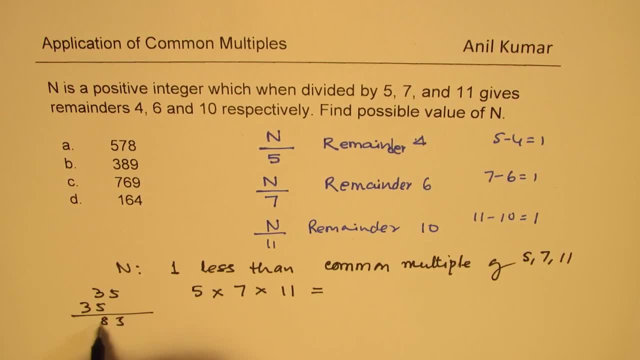 just add 35- 35, so you get 385, right, so it is 385. so we are looking for answer which should be not 385, but minus 1, which is 384. however, we do not have that kind of a number here. we have 389. now what to do? that's the question. 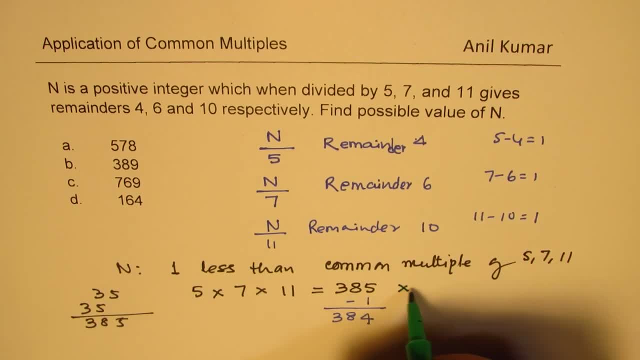 so now we have to try the next multiple, right? so the common multiple times 2 is what? let's multiply this by 2. so if I multiply this by 2, 5 times 2 is 10. double of this number, basically 16 and 117: 1, we get 770. now from 770, which is again a common multiple, will take away 1 and